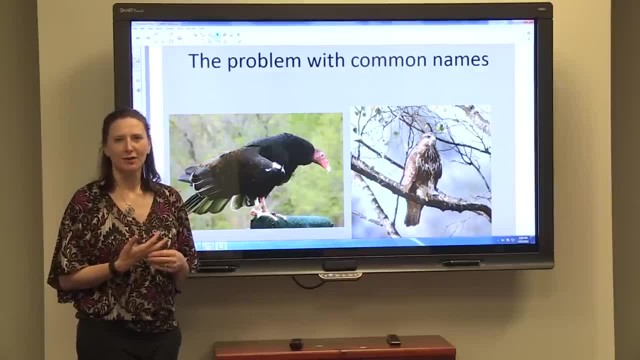 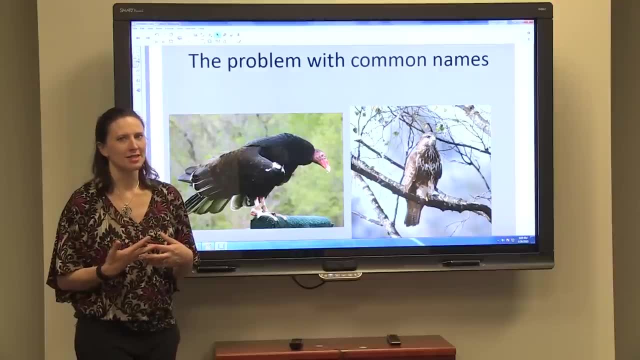 under false pretenses and that they were going to soon find out that I couldn't identify birds, because I was looking at those same birds and I wasn't seeing a buzzard. I was seeing what I would call a buteo, which is this bird. 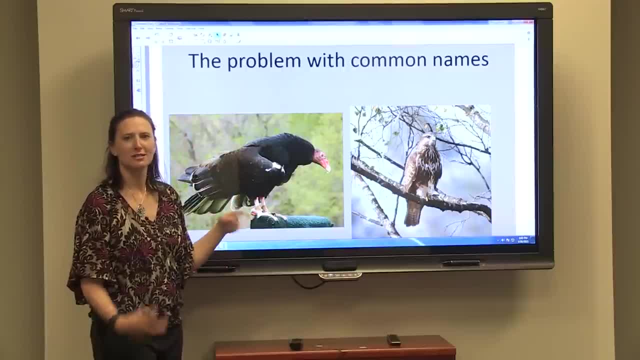 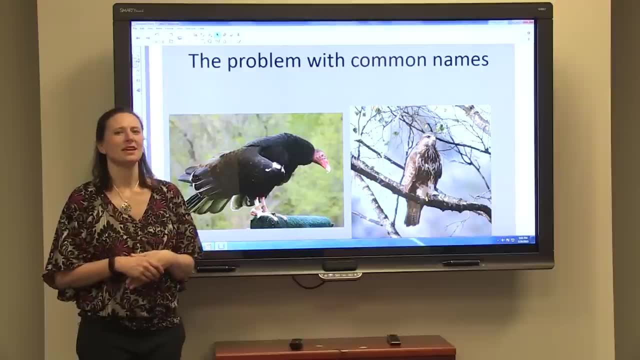 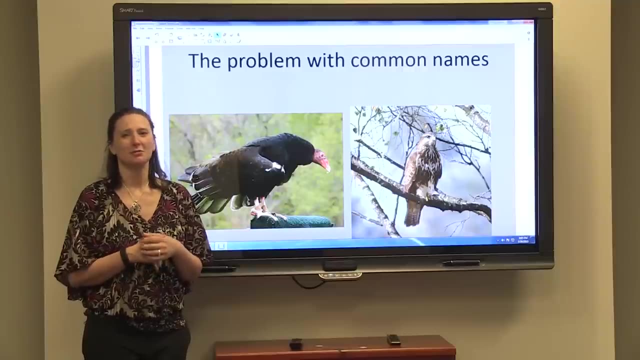 What I was thinking was a buzzard. A turkey vulture is also sometimes called a buzzard here in America. So I finally said to them: Um, can you show me what bird in this field guide you're calling a buzzard? Because I really was so confused and thought I didn't know. you know what birds I was. 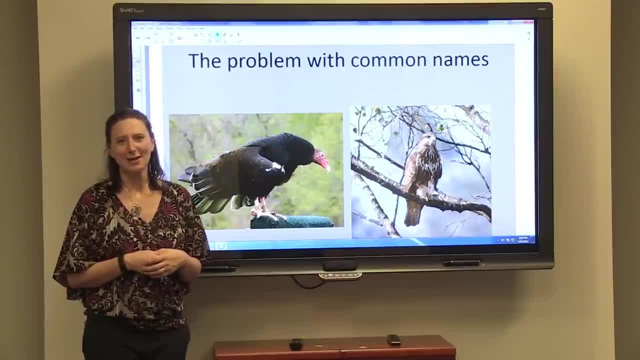 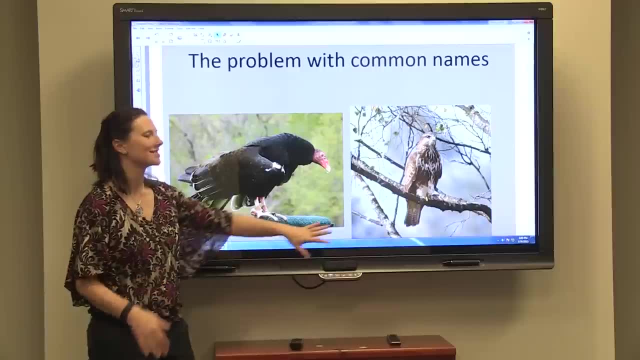 looking at I didn't know up from down, and that they were going to find out I was a scientific fraud and send me back to America. And so finally, it just became obvious that they called buteos buzzards, So their common name for this bird was a buzzard. 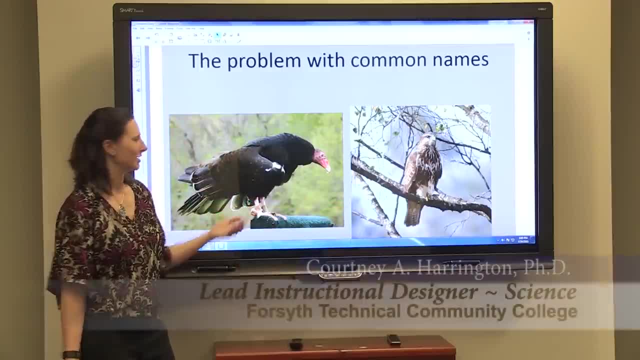 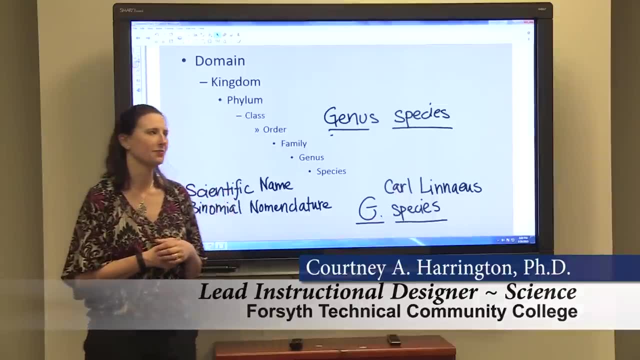 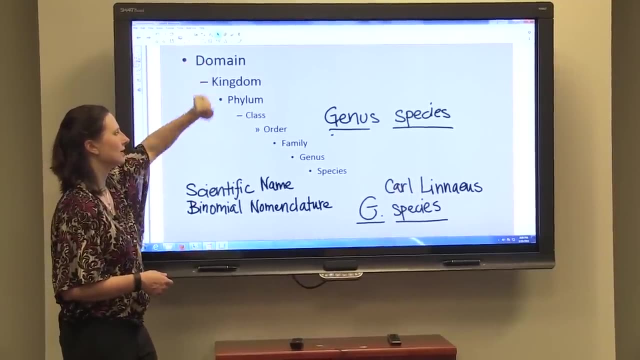 And that's what I was looking for, But they would have just called this a vulture or a turkey vulture. So, in order to have a naming system, we have to be able to classify organisms, And we classify organisms according to this domain system. 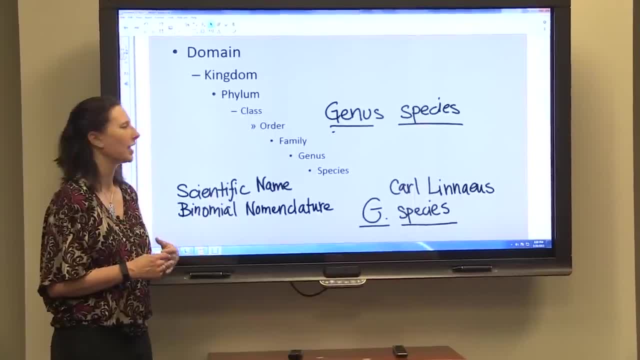 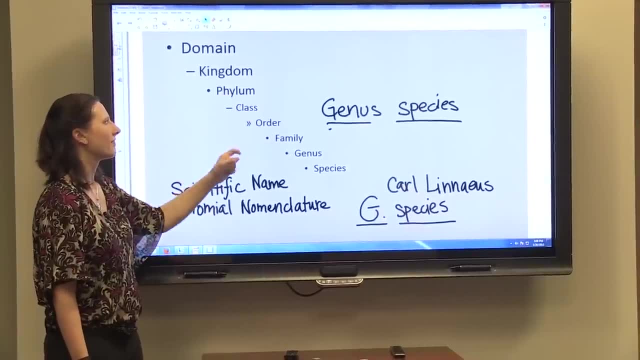 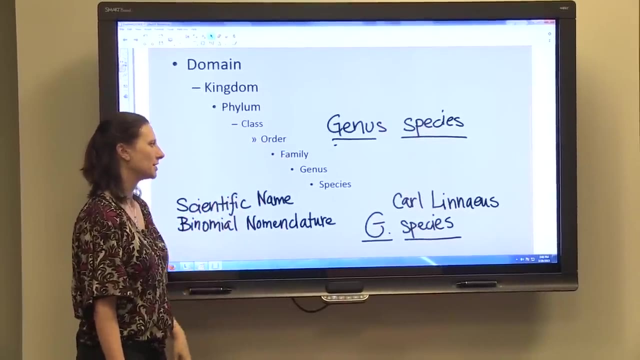 There are three domains: bacteria, archaea and eukarya- And within those domains, there are five kingdoms. Within those kingdoms, there are phyla. Within those phyla, there are classes. Within the classes, there are orders. Within each order are families. 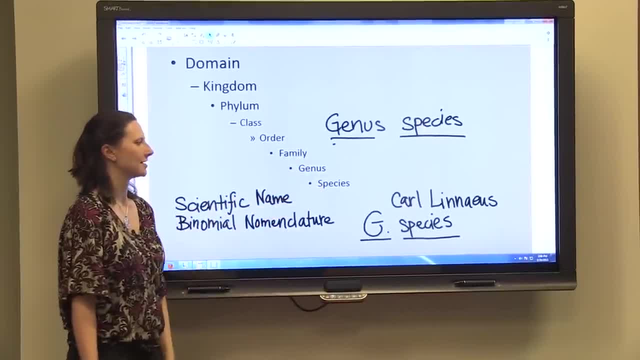 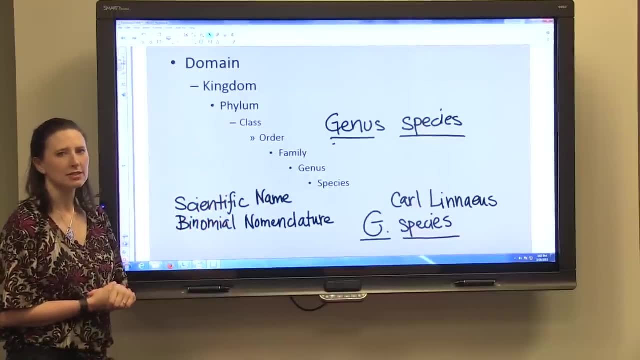 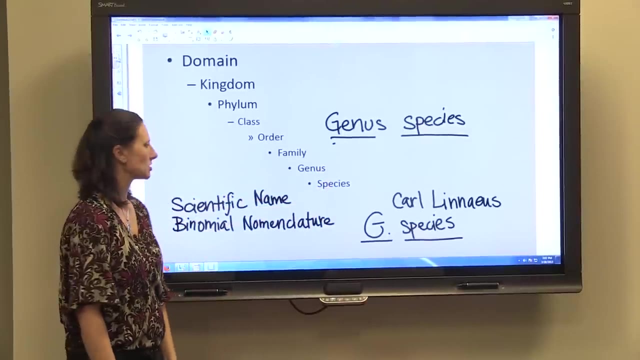 Within each family is a genus And within each genus is a species. So we can use this system of classification to differentiate between different species of organisms, because they will each have a unique combination of these classifications. So Carl Linnaeus, who was a Swedish scientist, came up with a system of binaries. 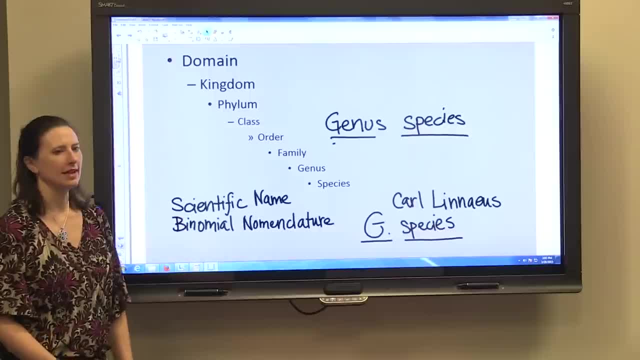 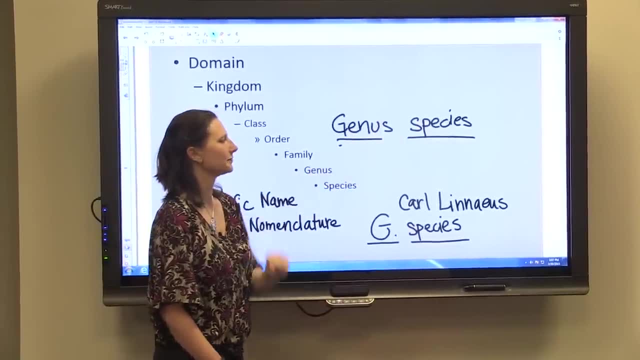 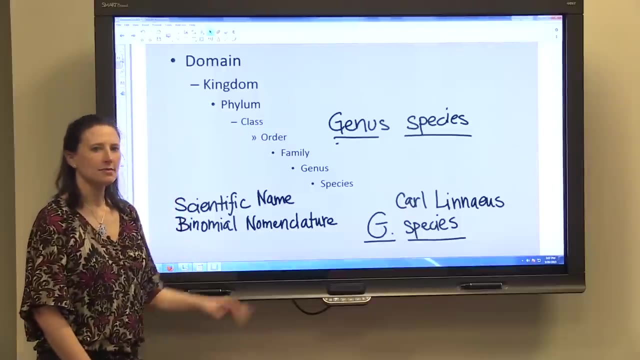 He came up with a system of binaries, which is called a binomial nomenclature, to determine scientific names, And that is that each species should be named, called by its genus and species Genus is always capitalized, The species is always lowercase.